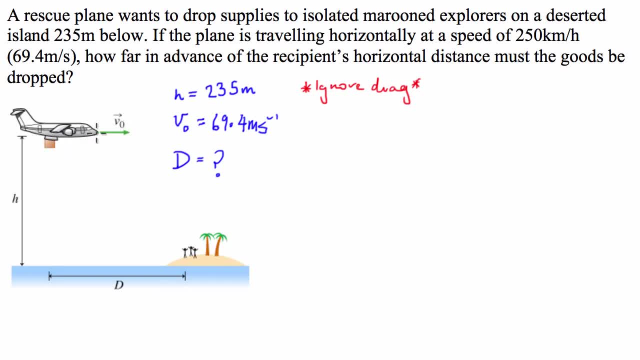 falls, it will accelerate because of its mass towards the ground, obviously, And it will take a sort of a parabolic motion. You'll start to see. it do hopefully do this Penetration. So what happens is, as the thing falls, the vertical component of its velocity becomes a greater proportion of its horizontal component and it starts to fall downwards at a faster and faster rate. 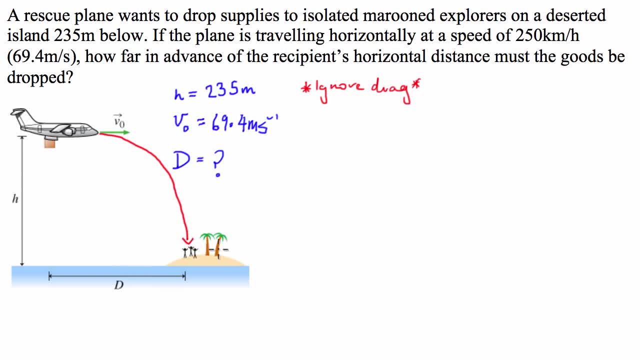 So how are we going to do this particular question? Well, to find d. I do know that the plane is flying and, as a result, the box will be flying in this direction at a particular speed. Now, what I need to do is I need to calculate, to start with, how quickly or how long it's going to take the box to fall through the height that we've been given. 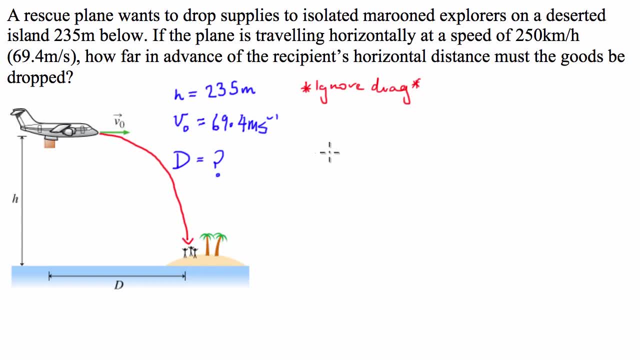 So we're going to go about solving that first. So we're going to use one of our equations of motion. So the first equation we're going to use. This is: s is equal to ut plus half at squared. Now what's good about this equation is it relates distance and acceleration in time. 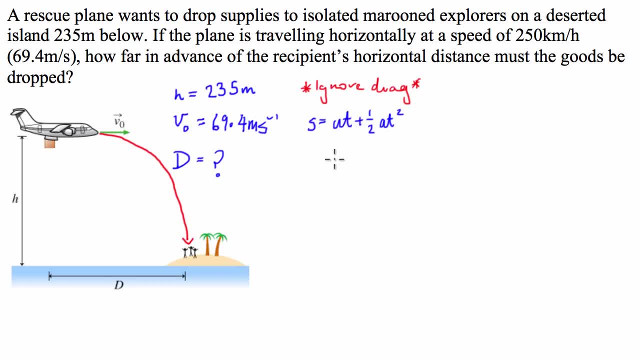 Now what's good about this equation also is that the initial velocity u is zero, So it basically cancels out half of it, So it makes it a lot easier to compute. So let's put in what we know. We know that s is going to be 235 meters. 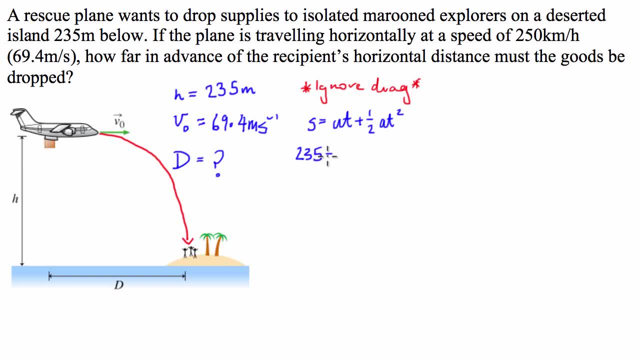 It's got to fall through Is equal to zero times time. So that's going to be zero plus one half 9.8, one times the time squared. There we go. So what we're going to do is we're going to rearrange this equation. 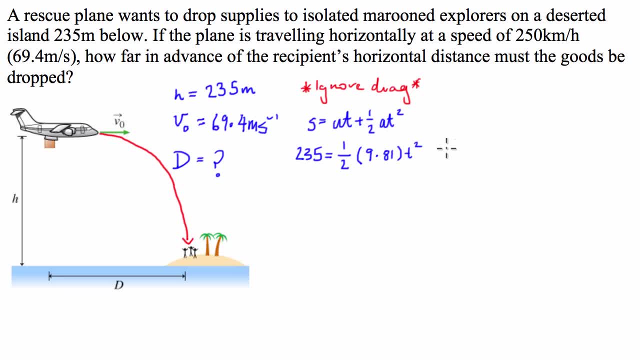 By moving the half across, dividing by 9.81 and square rooting, So we're going to end up with. t is equal to the square root of 235 divided by one half of 9.8.. 1. Cool, And the time is going to be 6.921 seconds. 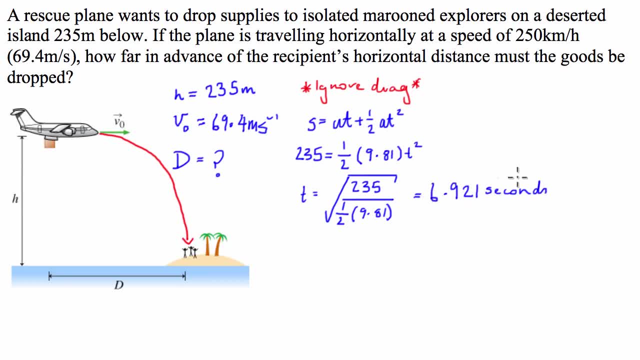 So that's how long the box is going to be in the air for. But what we then can do is, if we know that it's going to be in the air for that long, we have to figure out how much horizontal distance it's going to cover in this time. well, we know that the horizontal velocity 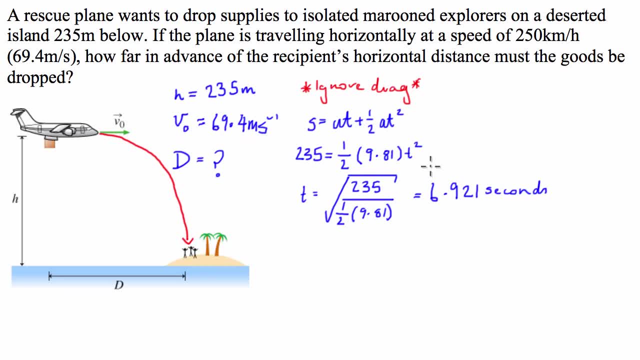 is 69.4 meters a second. we know it's going to be doing that for 6.921 seconds, so we're going to use- we'll just use the standard. distance is equal to velocity times. time or displacement is equal to velocity times time, which is equal to 69.4. 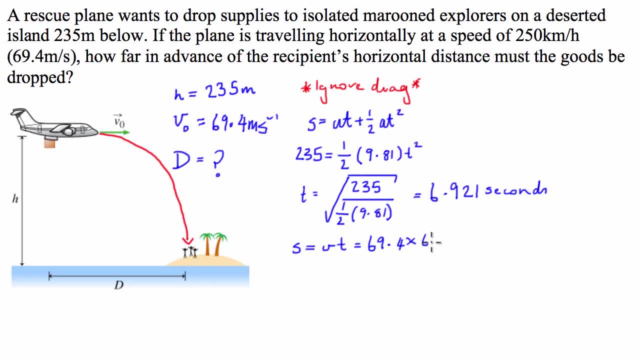 multiplied by 6.921 seconds. so what we can do is once we can just chuck that straight to the calculator and we get 480 point three, two meters. so what we know is that in this 6.921 seconds we're going to travel 480 meters. so it figures. 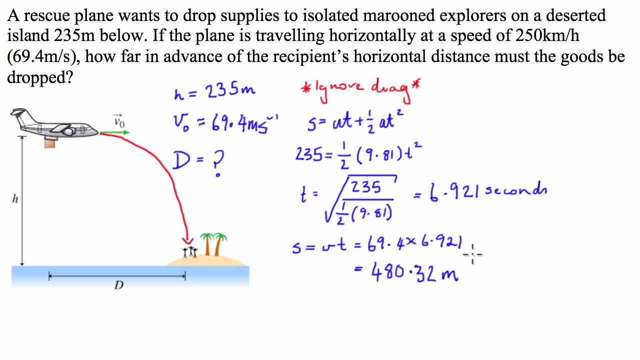 hopefully in your heads that if it's going to go this far horizontally, in that in the time that it takes to fall, surely we should then drop, throw the box out of the airplane or drop it out of the airplane 480 point three, two meters, the island. so the box, when it's lands, it lands on the island. so that's basically. 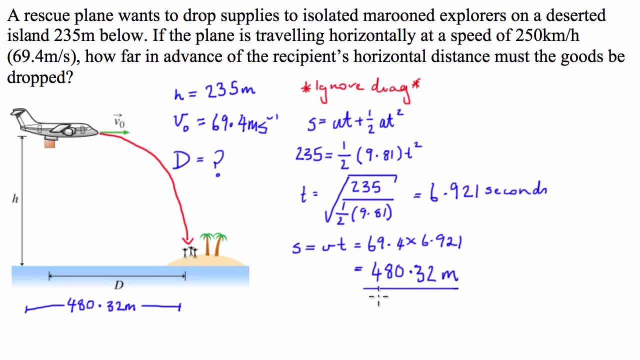 that answers this question, that is, our final solution- is 480 point three, two meters. so what we did to start with is we calculated how long the box would take to fall from the plane to the ground, all the while ignoring any sort of wind resistance. so there's not going to be any kind of terminal velocity or 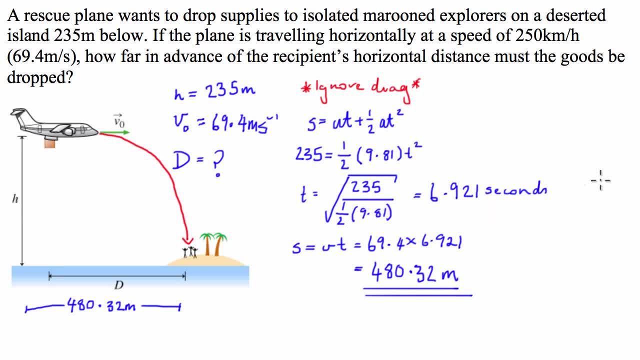 anything like that. what we then did is after we calculated the time, because we- hopefully you guys- understand that without drag, our horizontal velocity is constant. so if we know how long it's falling for and we know the speed of the airplane, we'll be able to know the distance in the horizontal direction. 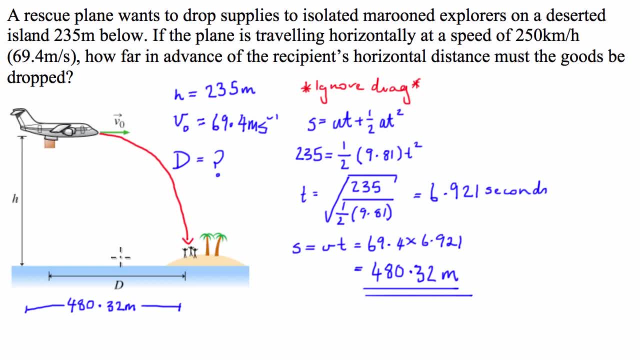 that the plane will be able to, or the plane and the box will be able to cover in the six point nine, two, one seconds. so if we just then we can just use the basic formula s equals V, T to calculate how far it's going to go in. 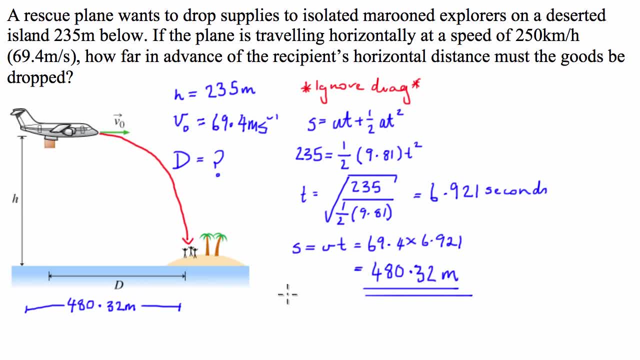 that time and, as a result, how far before the island the plane has to drop the box. so it's not a tricky problem, to be honest. I said it was easy to start with. hopefully that is easy for you, but again, I hope the video helped do us a favor. 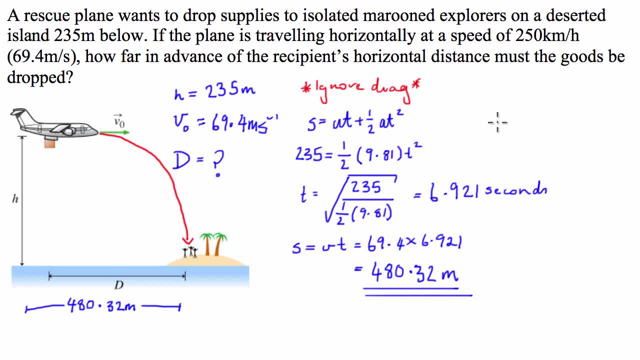 like my, like the channel or like like the video. sorry, subscribe to my channel. what are you thinking out? and hopefully, if you have any questions on physics, chemistry, maths, basically whatever, I'll give it a go at answering it. I'm always looking for a new challenge. so, yeah, hopefully I get some questions from you. and I'll see you again next time. 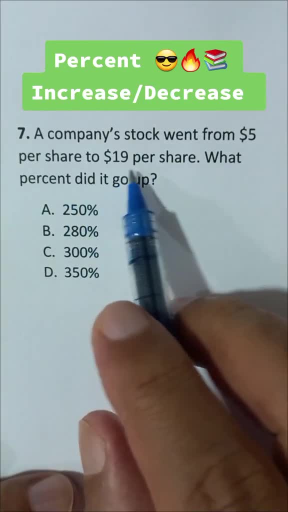 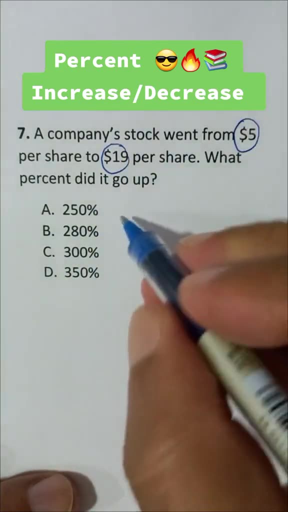 A company's stock went from $5 per share to $19 per share. What percent did it go up? First we take the difference of 19 and 5. It's 14.. 19 minus 5 is 14.. Then we put the original.